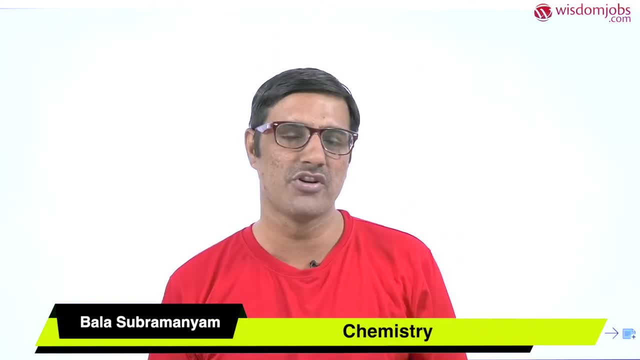 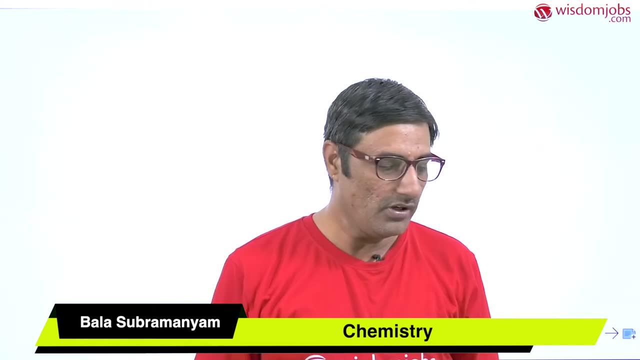 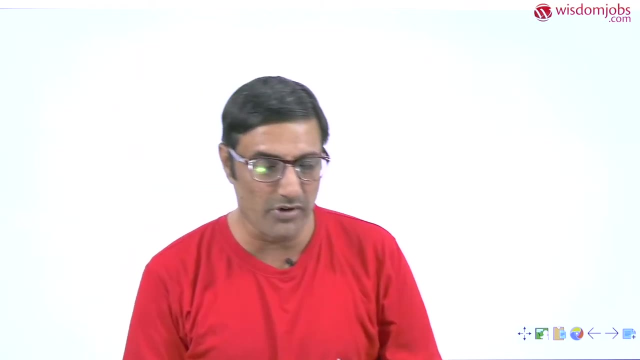 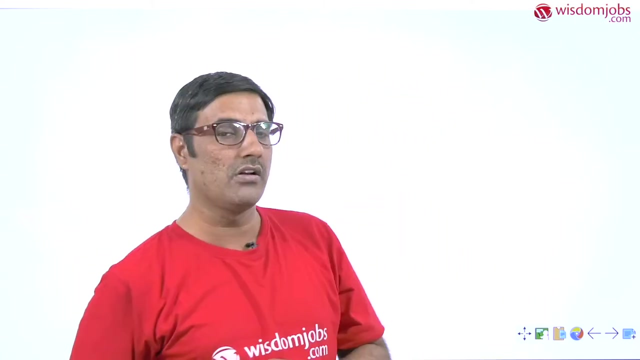 Hello everybody, a very warm welcome to all the viewers of wisdomjobscom. In this video I am going to explain you the conversion formulae from one coordinate system to other. So before going to start this topic, I once again request you all: please do subscribe to our channel, wisdomjobscom, and please do share our videos, because they are very, very important and very useful also. So we are going to cover all the basics so that you can use these basics in the advanced topics and do some 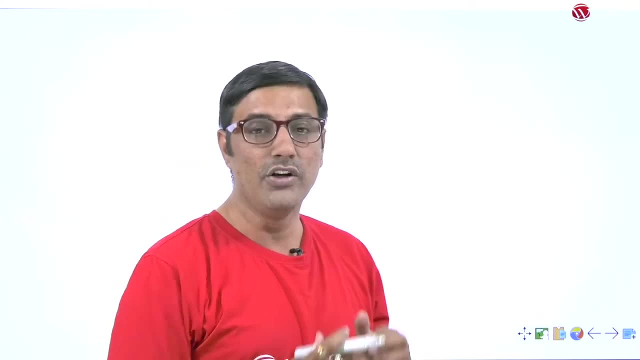 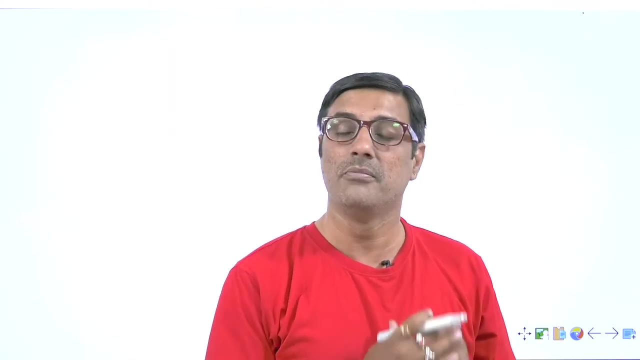 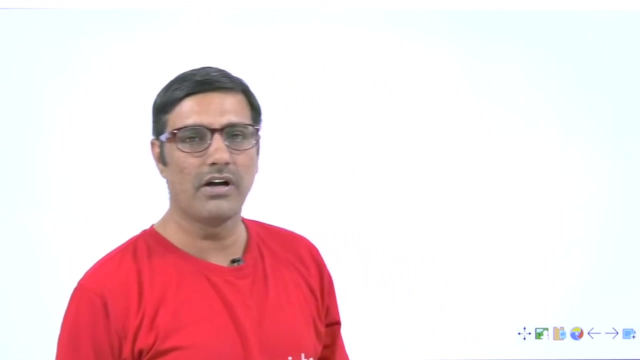 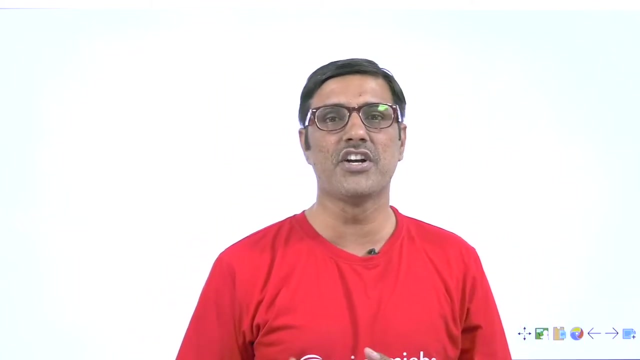 problems. So whenever we are doing problems, these basics are very, very useful for you, so that we are asking you to subscribe to our channel and if you find our videos to be informative, please do have a like. So with this note, I am going to start the topic Now. in the last videos, I have thoroughly explained about what are the different types of coordinate systems and also what are the parameters that are involved in each and every coordinate system. So in this video, let us start with the conversion formulae. Now, basically, 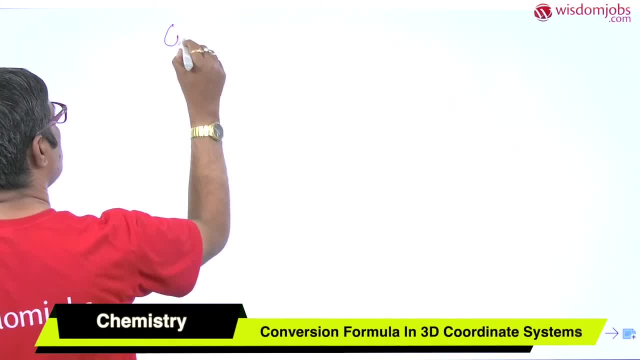 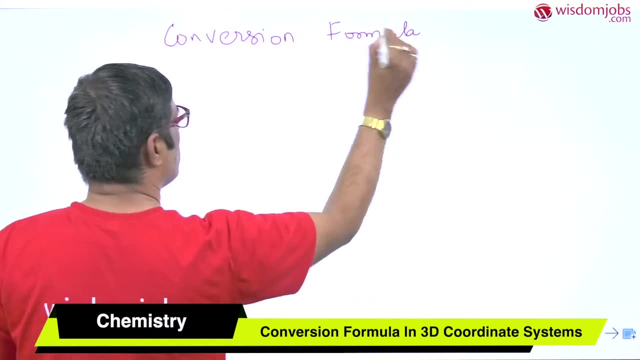 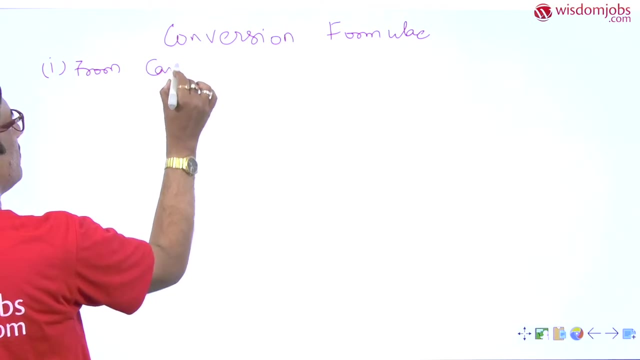 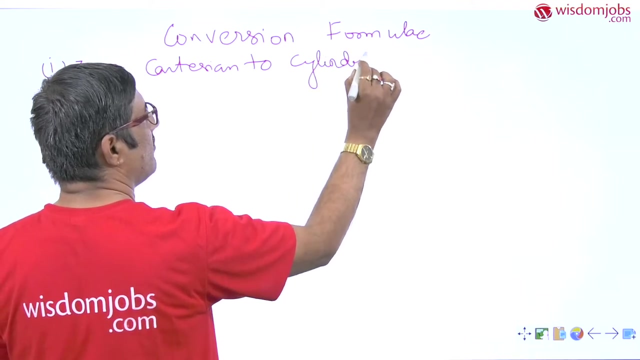 we have got two types of conversions. So one is conversion, So the heading is conversion formulae. Now here, the first variety is from cartesian to cylindrical. Now, what is a cartesian coordinate system? How we are going to represent a point here, It is a. 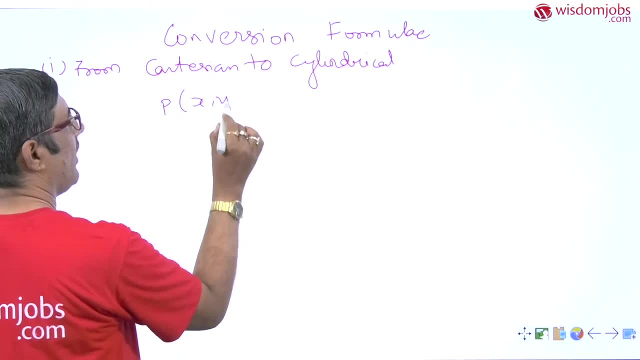 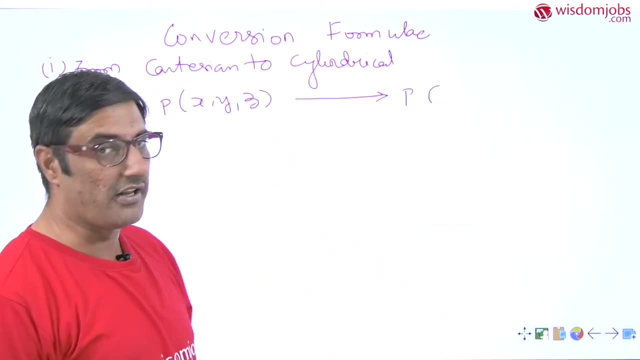 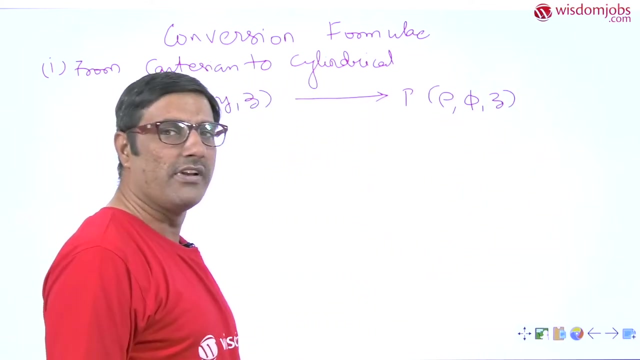 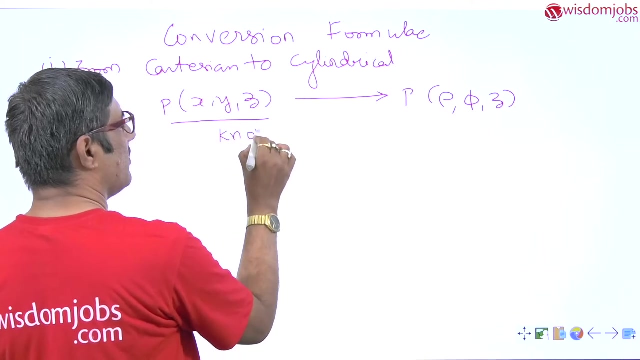 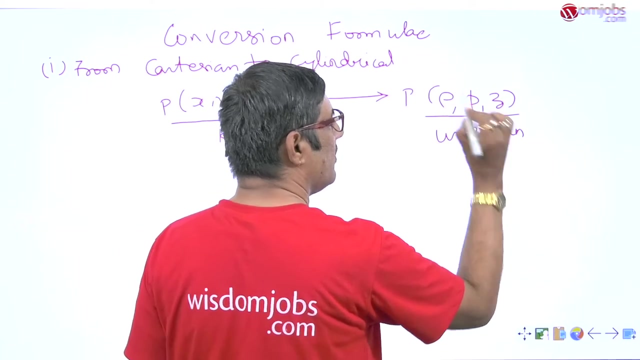 p of x, y, z to p of how a point is represented in cylindrical: it is rho, phi and z. So whenever I say cartesian to cylindrical means- this is known for you, Known are cartesian and unknown are cylindrical- That means I need 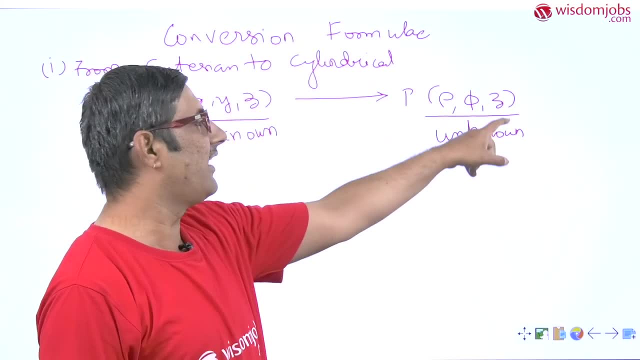 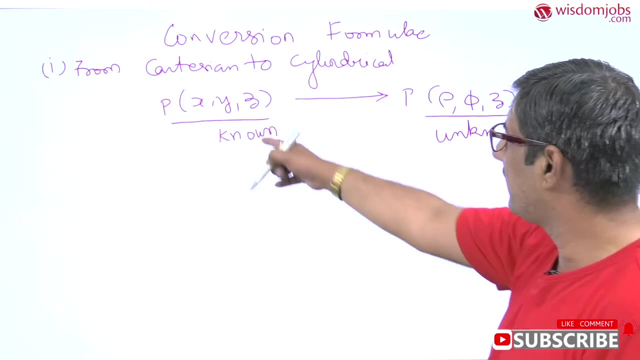 to write the formulae for rho phi and z in terms of x, y, z. ok, So rho phi and z should be known to you in terms of the given parameters or non parameters. So what is row actually? row is simply under root of. 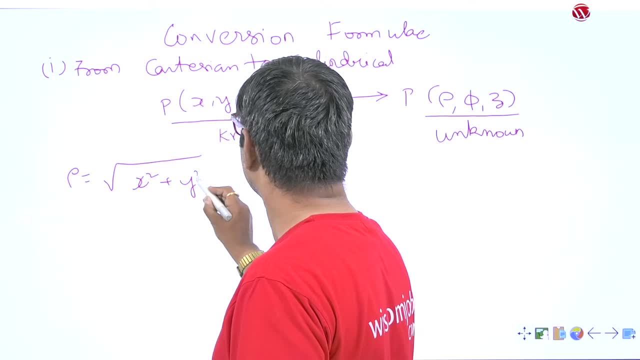 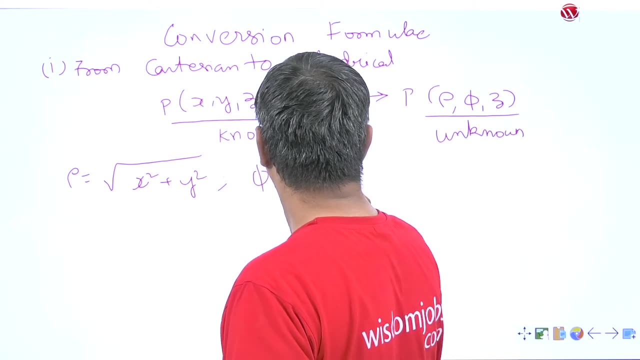 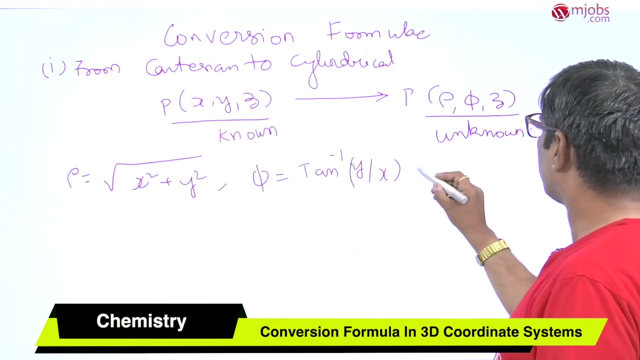 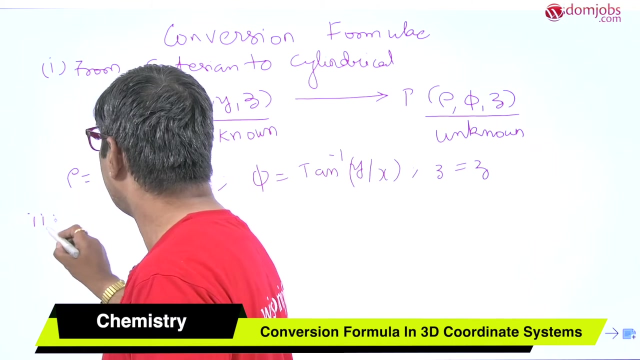 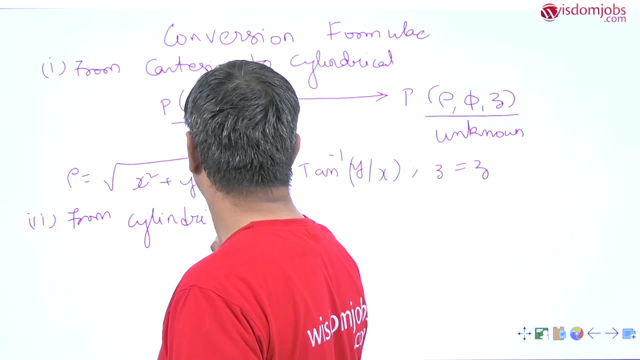 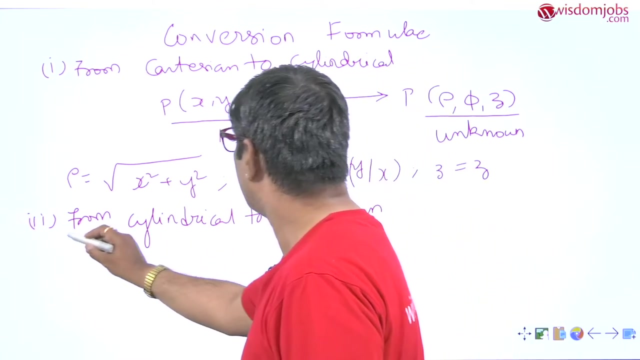 x square plus y square. This is the formula of a row. Next, what is phi? Phi is simply tan inverse y upon x. and what is z? Of course, z is z only. Next, second variety, if you observe, from cylindrical to Cartesian means, from p, what is cylindrical coordinate system representation? 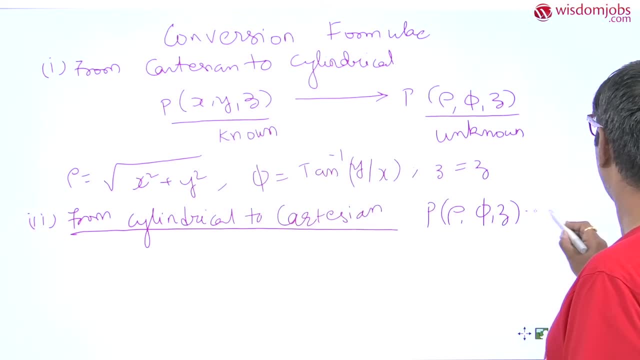 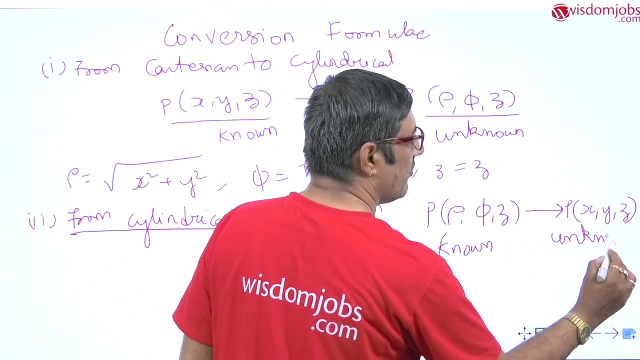 rho phi, z to p. x, y and z means you know this. So these are the known parameters for you. Rho, phi and z are known to you. and what are the unknowns there? x, y, z. So these are unknowns for you. So obviously. 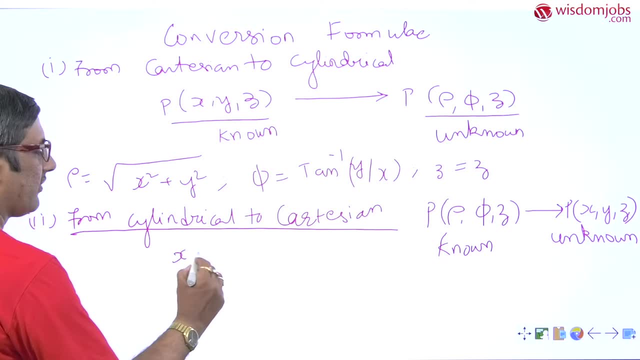 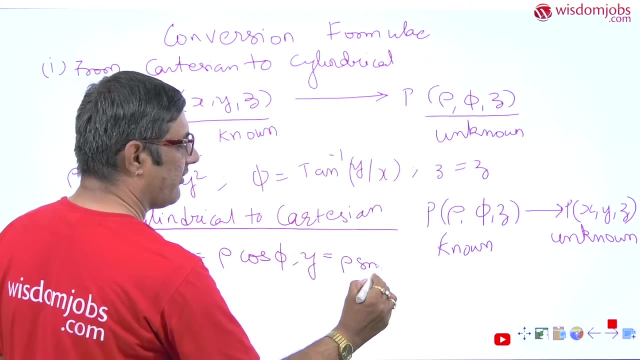 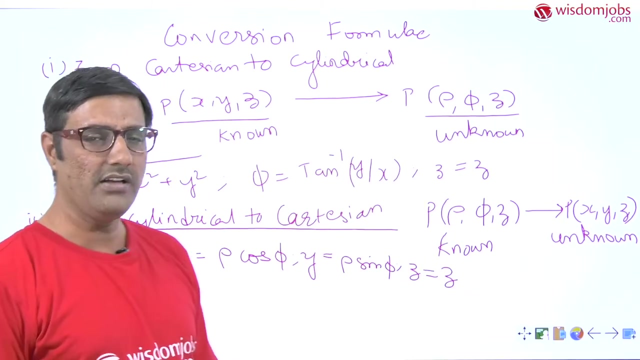 what is x actually? I can say: x is equals to rho cos phi, y equals to rho sin phi and z is z. So there is no change in z, but x is given by rho cos phi, y is given by rho sin phi. So these are the conversion formulae from one system to the other, including, I mean. 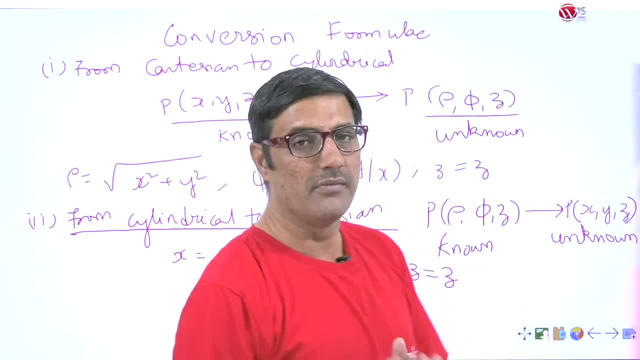 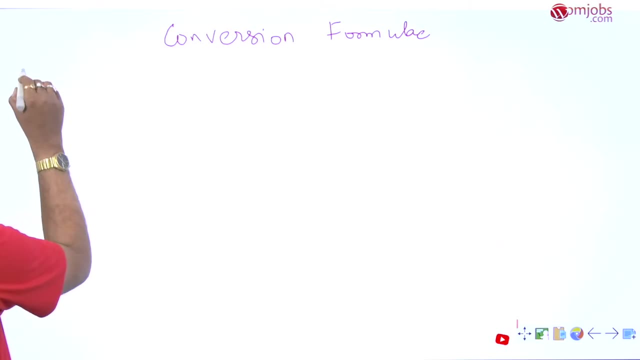 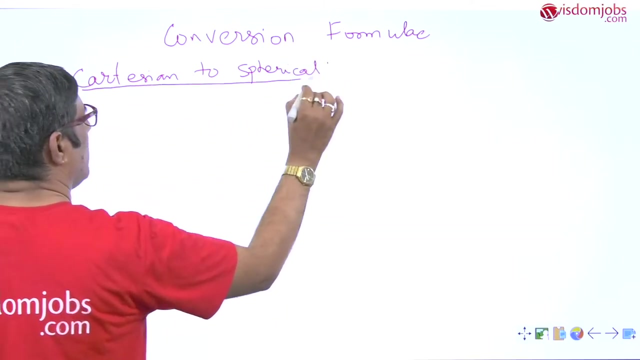 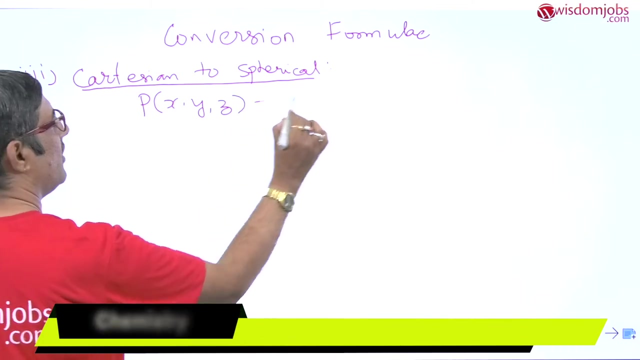 in between Cartesian and cylindrical. I mean, let me give the conversion formulae from spherical to Cartesian and Cartesian to spherical. So the third variety is, let me say, Cartesian to spherical. Okay, now, what is the representation of a point in Cartesian P, x, y, z, and what is? 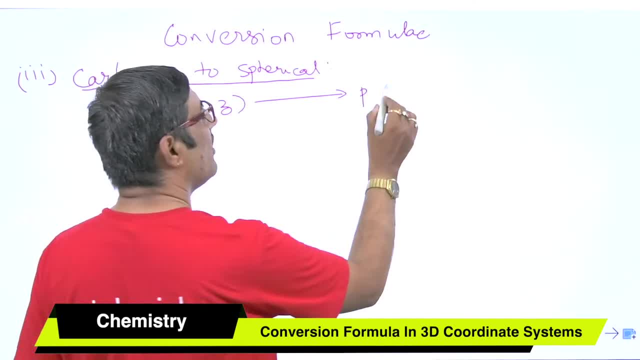 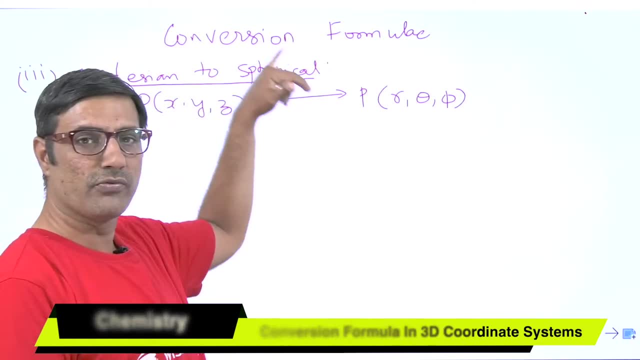 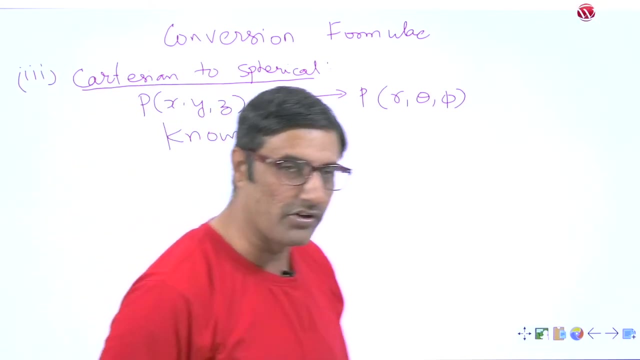 spherical coordinate system representation of point P, R, theta and phi. So if I am interested in getting spherical coordinate system values from Cartesian, I know them, I know Cartesian. So known values are what here? Cartesian coordinates values and what are the unknowns, The spherical? Okay, so that means that these are unknown. 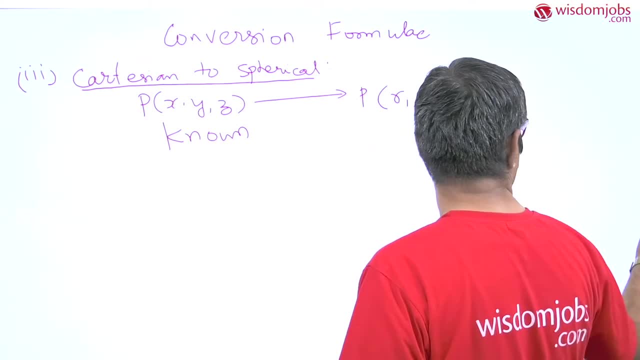 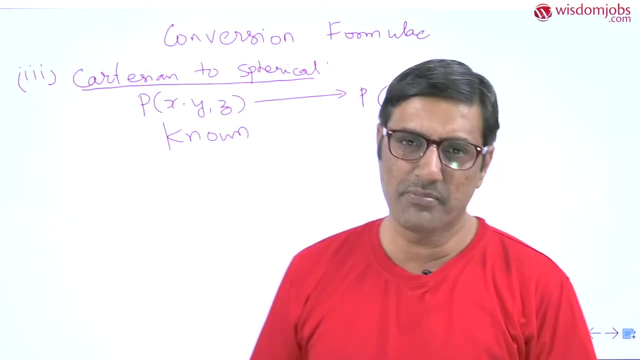 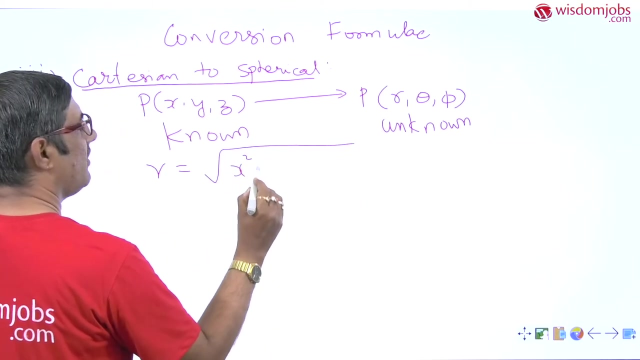 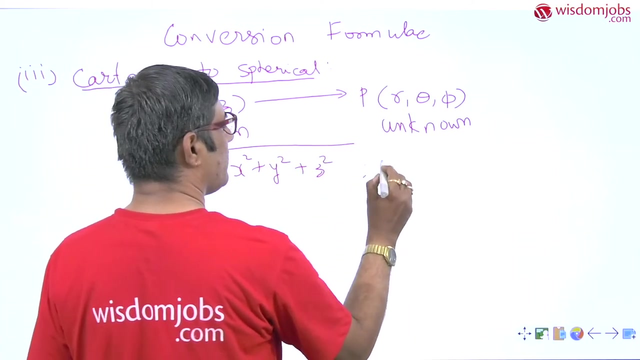 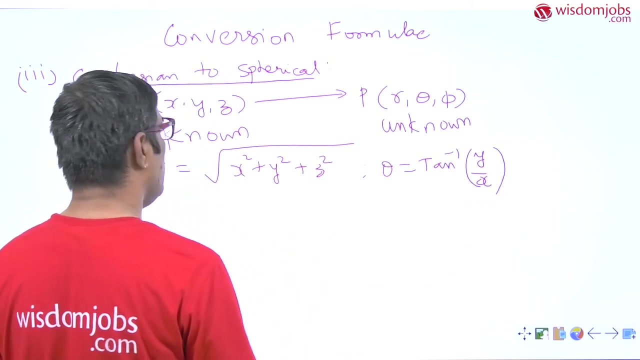 What are unknowns actually here? It is these r: theta and phi. Okay, now let me write the equations. So r simply under root of x square, y square, z square, sin sat. okay, and theta is tan inverse y by X. and what would be Phi? Phi would be cos. 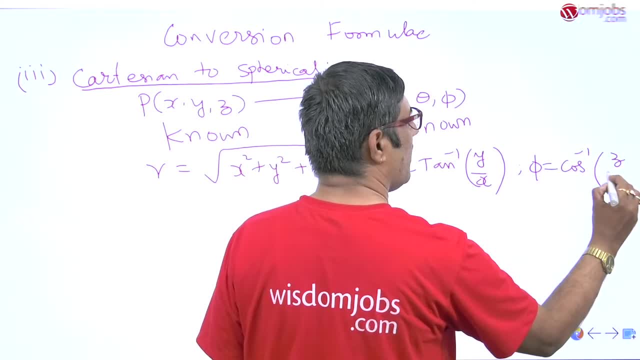 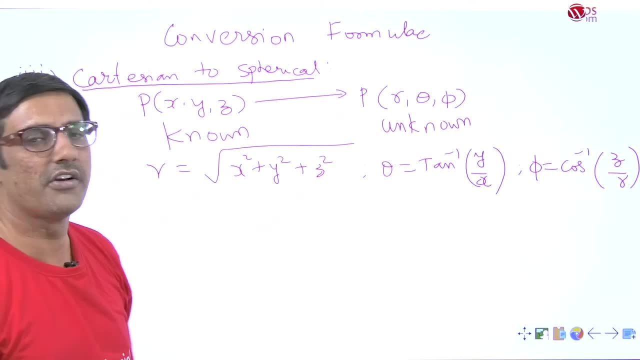 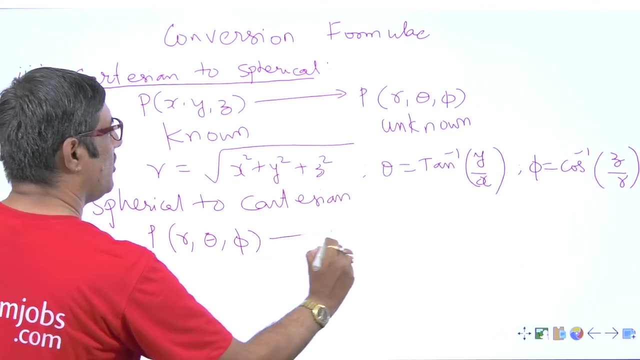 inverse z by R. okay, cos inverse z by R. so these are the conversion formulae from Cartesian to spherical coordinate system. now let me go for the fourth conversion formulae, which is spherical to Cartesian. okay, so our point is represented in spherical P, R, comma, theta, comma Phi to what is Cartesian. 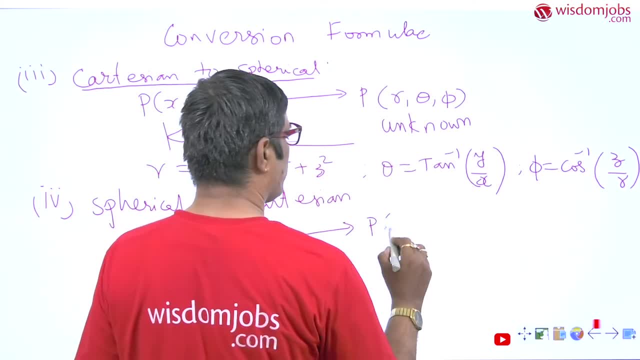 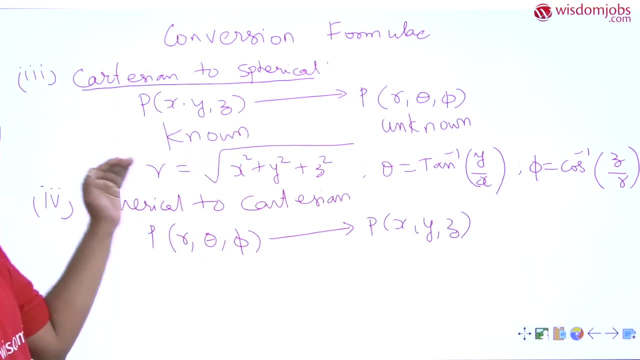 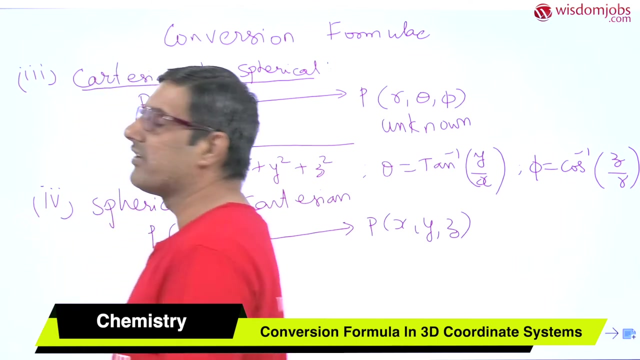 coordinate system representation of a point: P, X, comma Y, comma Z. so which are known here, how? which are known here how? which are known spherical to Cartesian means? we know spherical, so spherical coordinates are known for us. okay, spherical coordinates are known, and which is a? which set of? 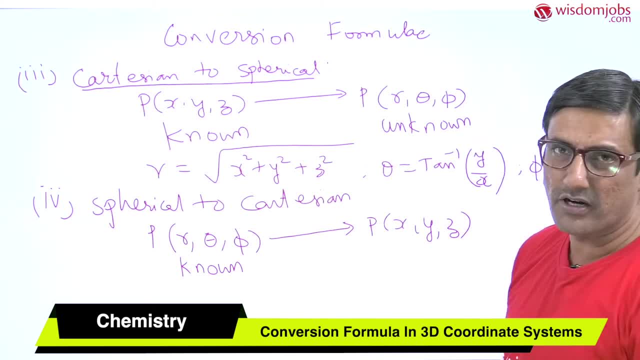 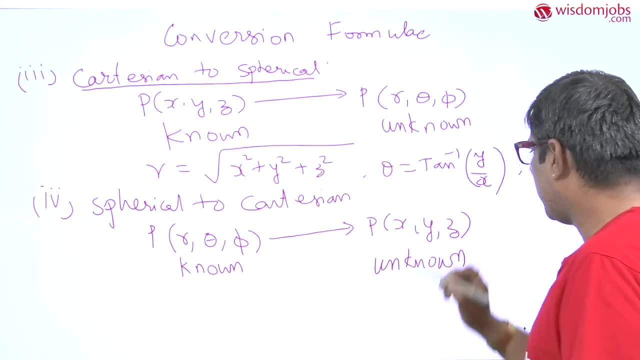 coordinates are unknown for us. it is the Cartesian coordinate systems, I mean Cartesian coordinate values. so these are unknown. so now let me write the equation for X, Y & Z. okay, so now all of us know the famous oscillator: Oh, SC. okay, why am I telling you this? because we are the only ones ever going to understand this. 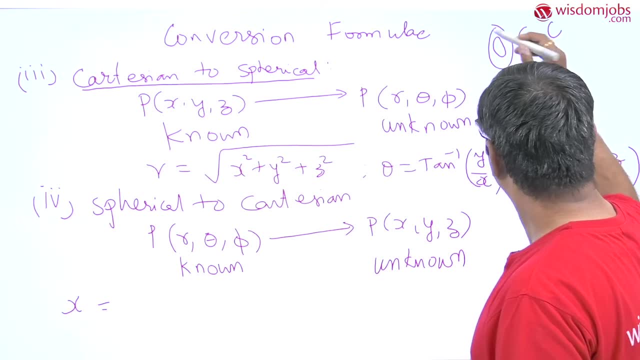 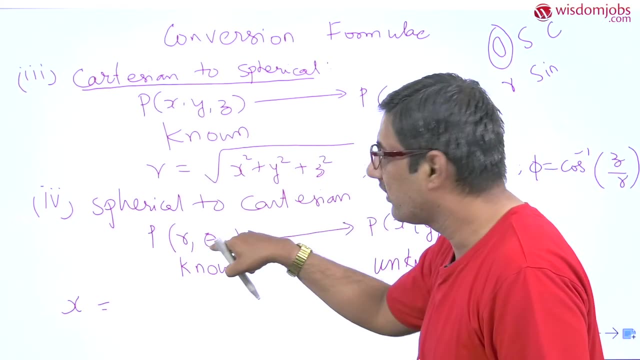 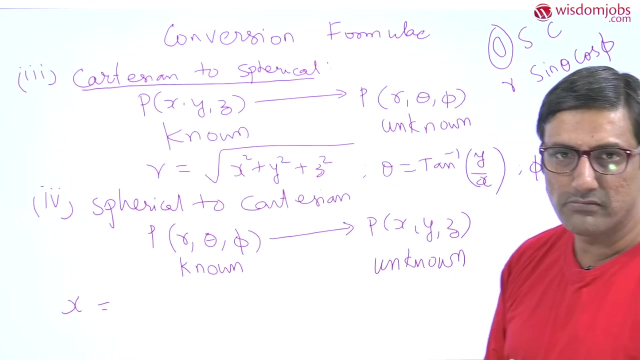 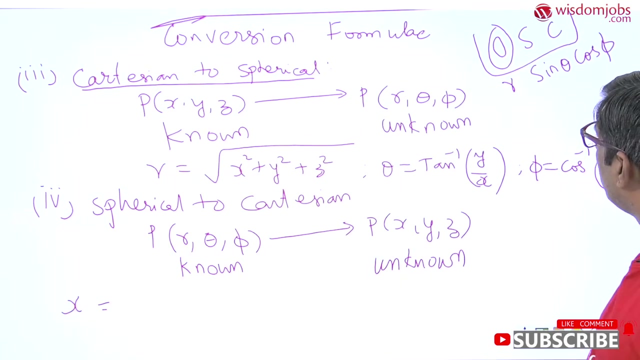 telling you all this here, because replace o with r and s with sine. and what is the first angle of the two here? theta, r, sine, theta and cos phi. okay, so the short form of oscillator we use in our electronics is osc, right? so if you remember this word, oscillator, then you can easily remember how. 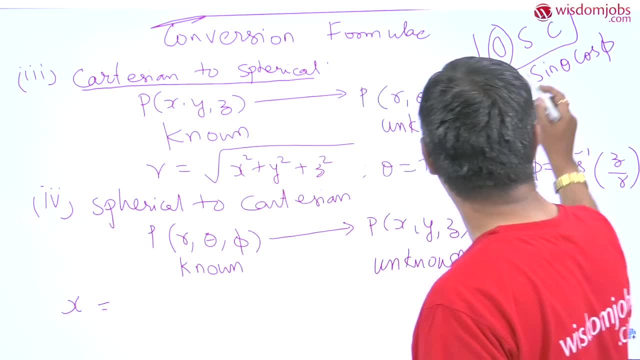 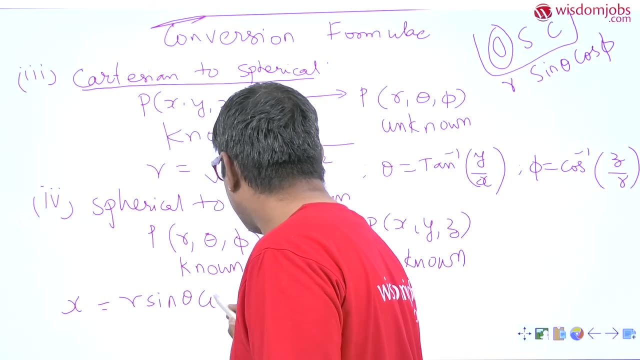 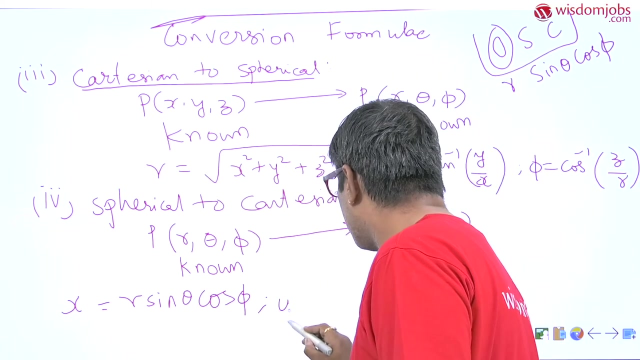 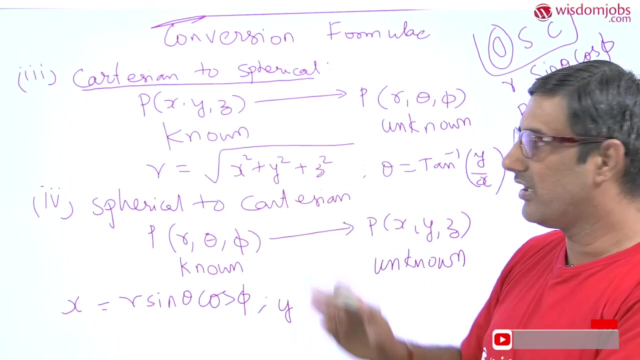 to get the expansion formula. okay, so r sine theta cos phi. so x is oscillator. so r sine theta cos phi, okay. next, if you go for y, so remember the word rss, so it is simply last year. so i am saying: okay, why am i telling you rss here? because y is r sine theta. 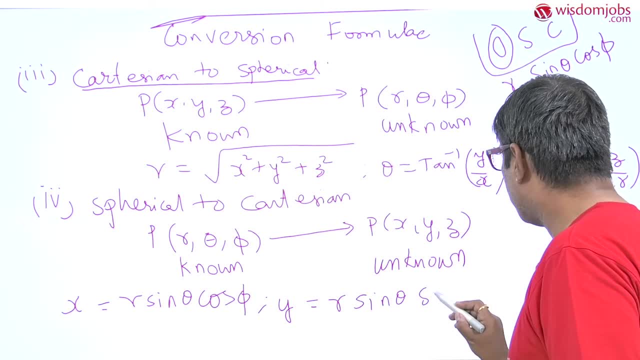 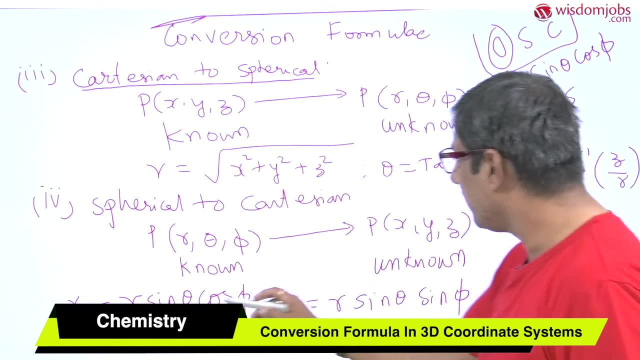 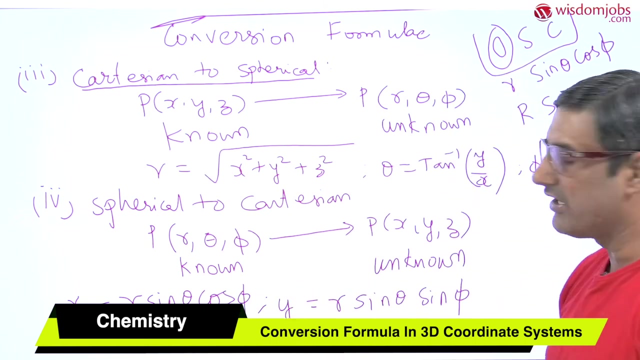 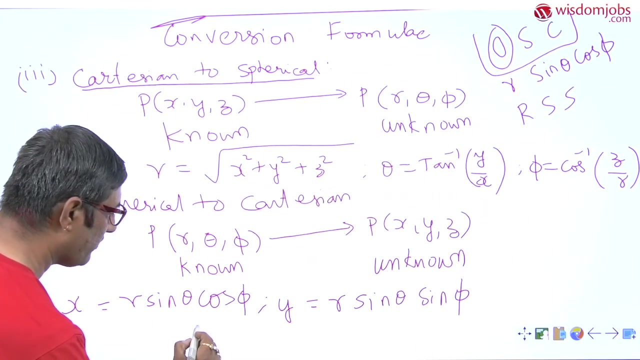 okay, sine phi, r, sine theta, sine phi, right. next, what would be now here? sine theta and sine theta, both are common here. okay, so here you have got cos phi and here you got sine phi, right. so how to get now the third parameter, which is z? actually, now, z is simply replace, of course, r would be as it is. 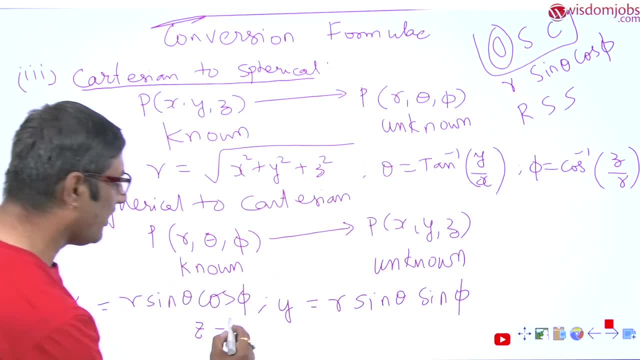 so in both the cases you have got sine theta. okay. so here you will be got getting r cos theta, okay. so in this way now, since sine theta is involved in a axion by both, there is no cos theta involved in any of these two formulae. so that cos theta is. 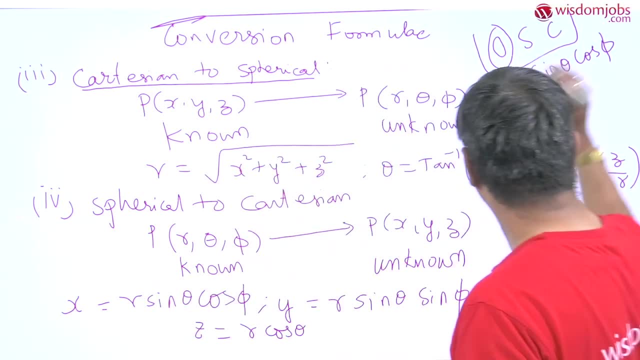 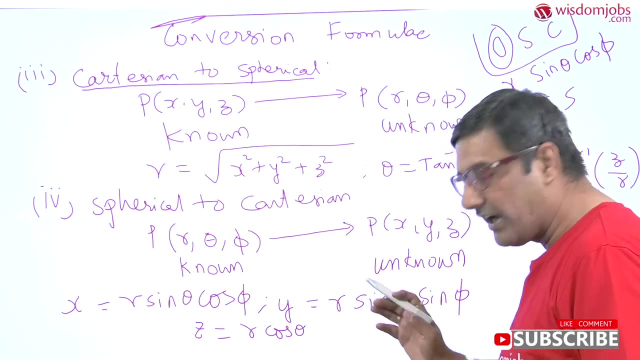 made involved in z. so if you remember oscillator, you get x, if you remember rss, you get y. and since in both the cases sine theta only is involved and cos theta is not involved, cos theta should be involved in z, so z is given by r, cos theta. 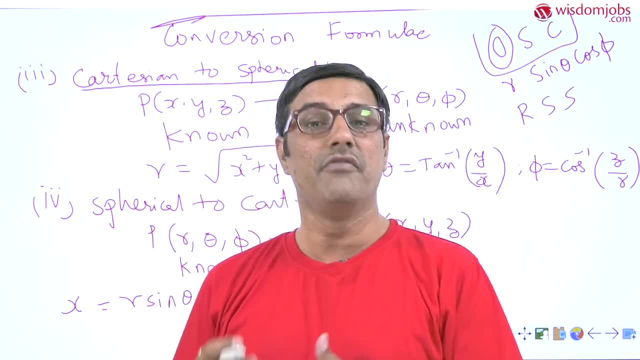 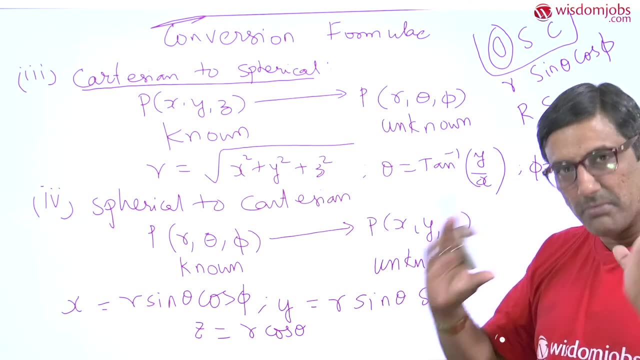 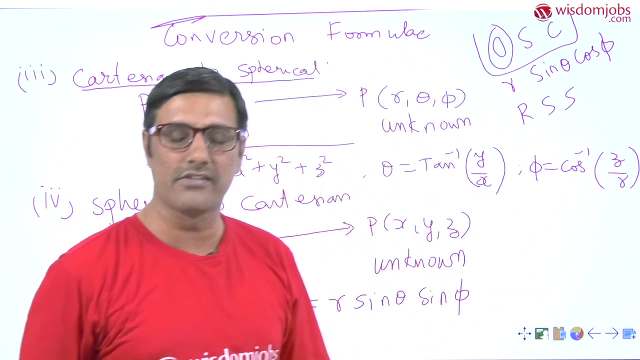 So in this way, you can easily remember the conversion formulae, which are otherwise very confusive and difficult to understand. okay, So you can easily comprehend and remember or memorize this formulae by the words oscillator and RSS. okay, So do not forget these two words, RSS and oscillator, so that they are very helpful in remembering. 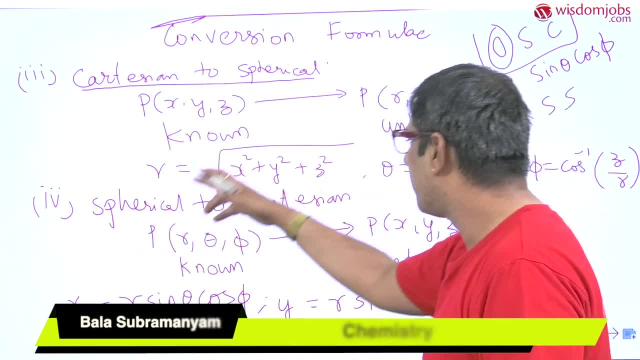 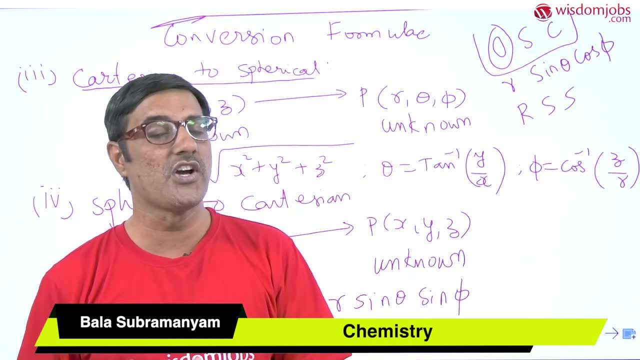 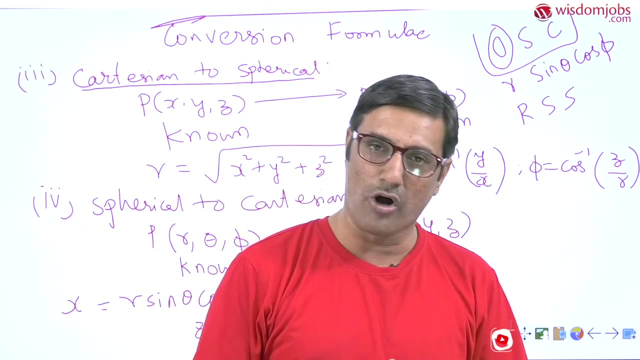 the conversion formulae from spherical coordinate system to Cartesian coordinate system. So with this note I am ending this topic. So please do subscribe to our channel so that you will be very much benefited and these videos are very much useful for you for the forthcoming topics.